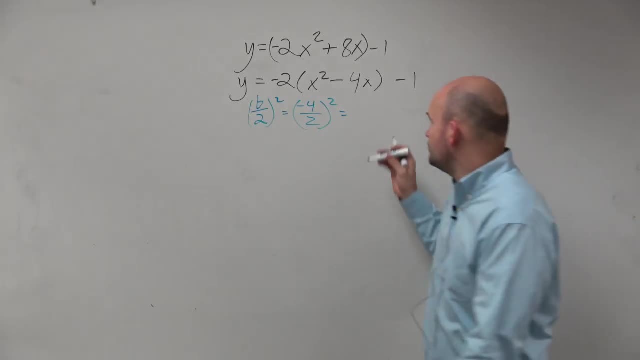 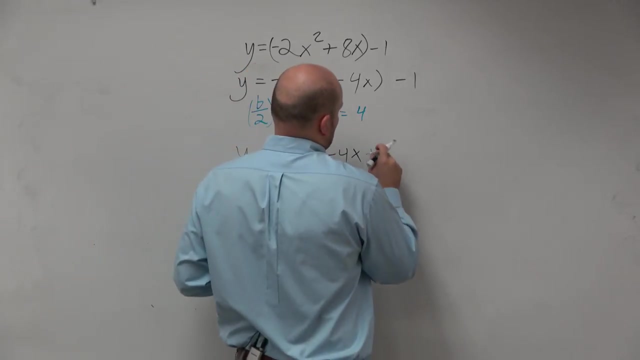 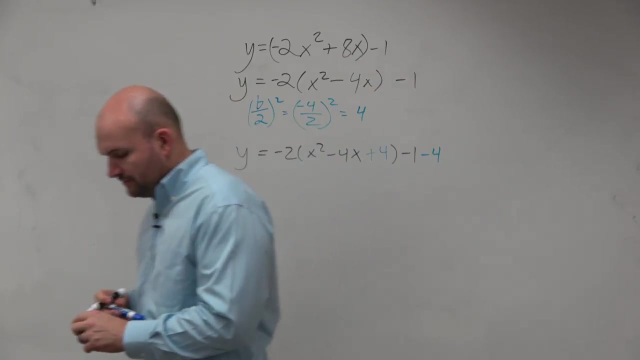 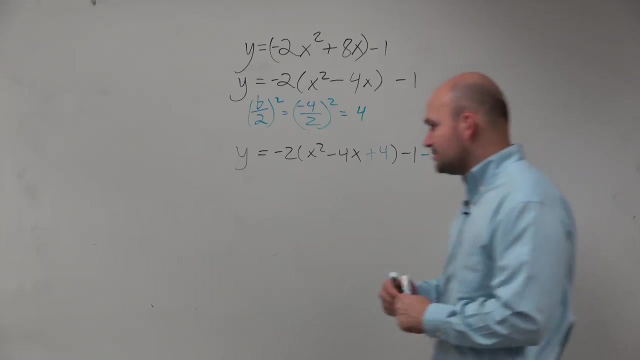 squared. Negative 4 divided by 2 is negative 2.. Negative 2 squared is equal to 4.. Add that Okay. So hopefully you guys get to this point. But then we need to kind of elaborate on something. Ladies and gentlemen, let me ask you a question: Are these two equations equal to each other? 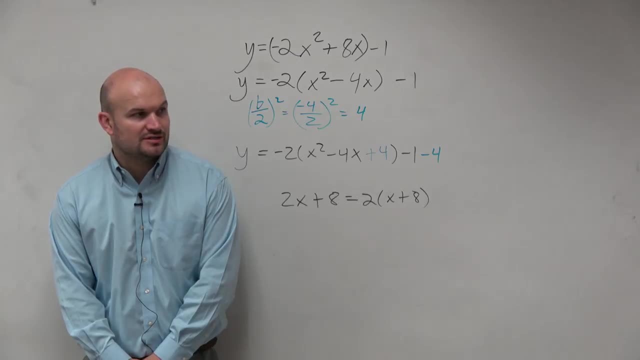 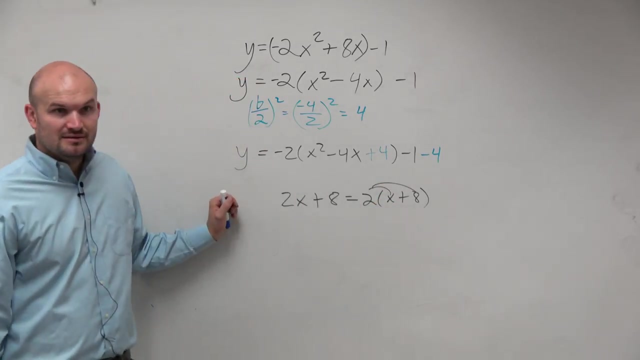 They're not equal. Why are they not equal? Somebody give me a justification. Yes, Princeton, Because you're the one taking 2x plus 16.. Yeah, This one. yeah, The Street of Property applies right. This is obvious, Does everybody? 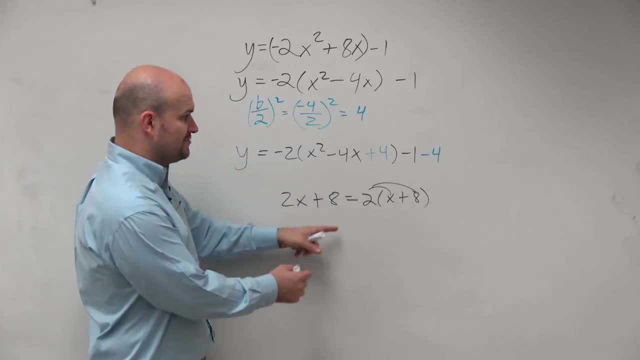 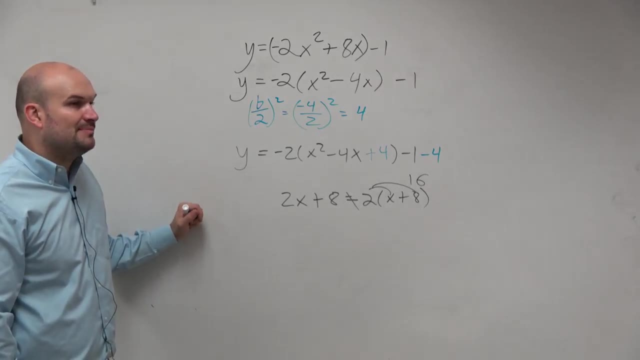 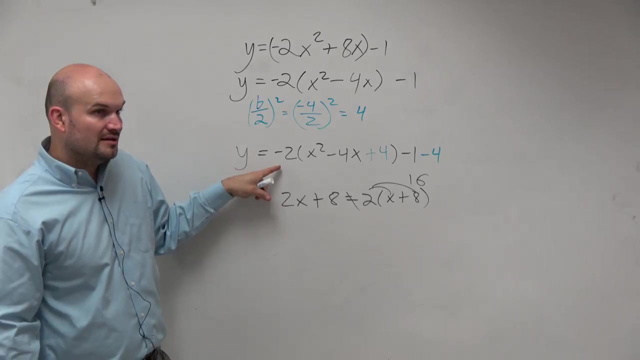 agree with me. That's kind of everybody understands that this is really not equal, because really that ends up being 16 when you multiply them, right? Well, guys, it's the same thing. This is not true. This 4 is really being multiplied by a negative 2.. So you're not adding 4 and 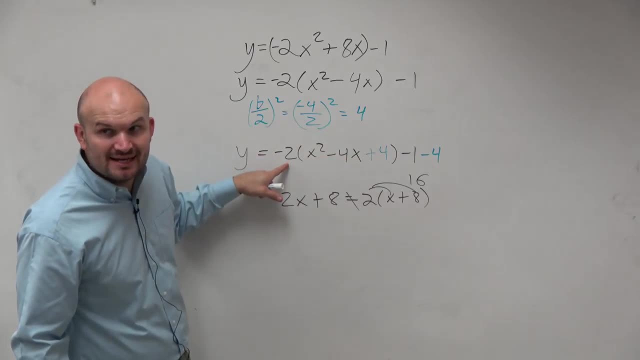 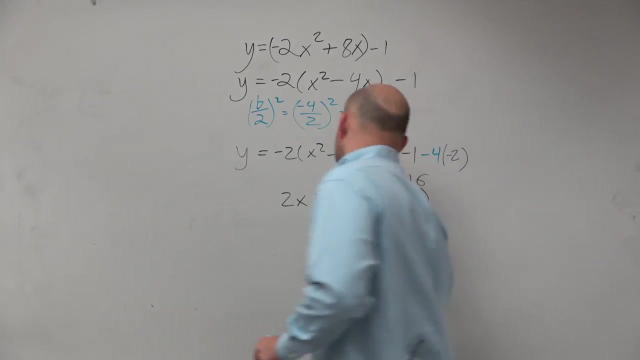 subtracting 4.. You're adding a 4 that got multiplied by a negative 2.. You're not adding by negative 2. So you have to subtract a 4 that's being multiplied by negative 2.. Really, really important stuff. 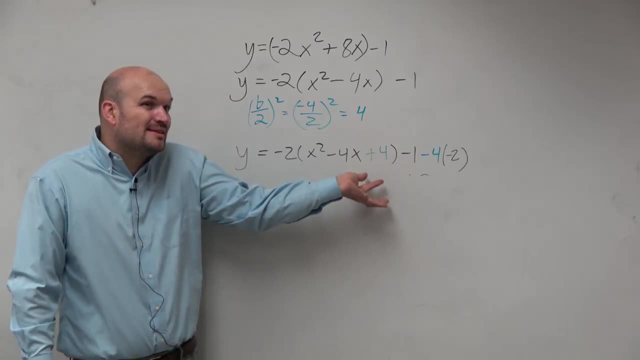 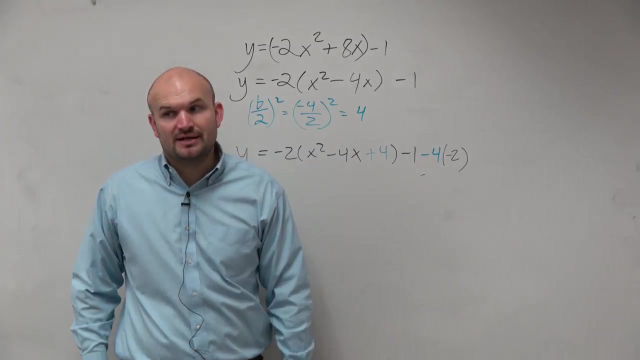 But does that make sense? You're not adding 4.. That 4 is inside parentheses. that just got multiplied by a negative. that are multiplied by a negative 2, Zoe. So therefore, when you subtract a 4, you got to make sure you multiply that by negative 2. 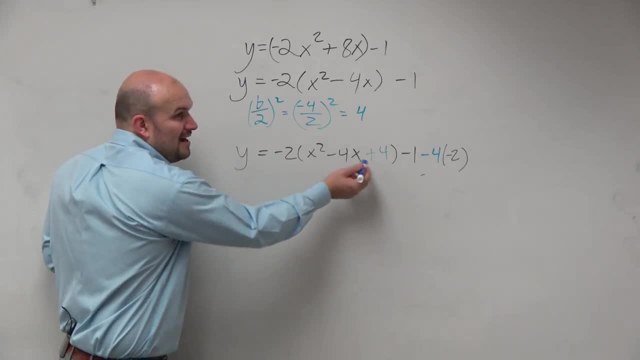 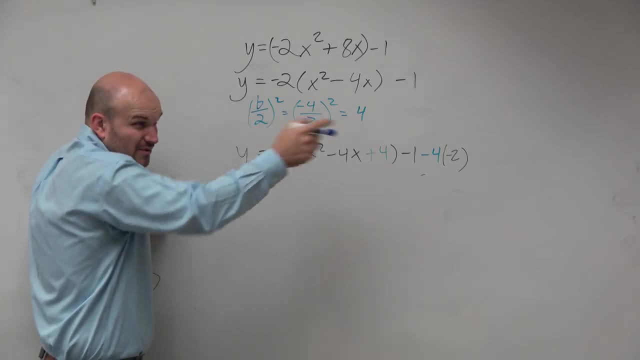 as well. All right, Now again, is this a binomial, squared, Is it? Is it a binomial? I'm sorry, Is it a perfect square trinomial? Does it look like the one that we already did in our warm up? 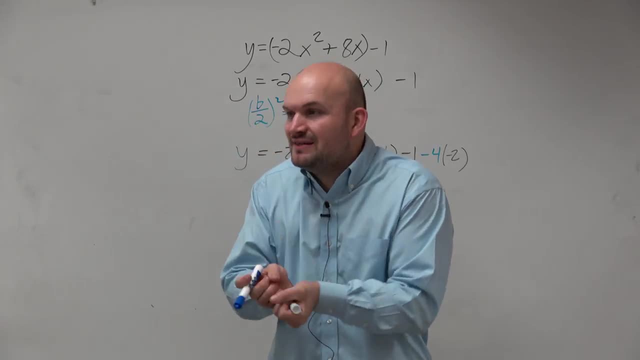 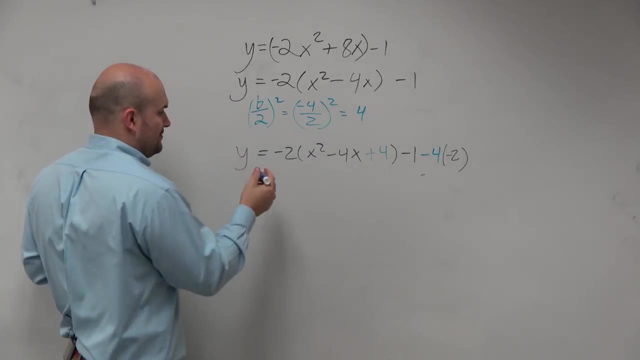 Yes, Every single time. I'm going to tell you guys, you don't even need to think about this. Every single time you do this, you are creating a perfect square trinomial. It's going to factor to a binomial squared. 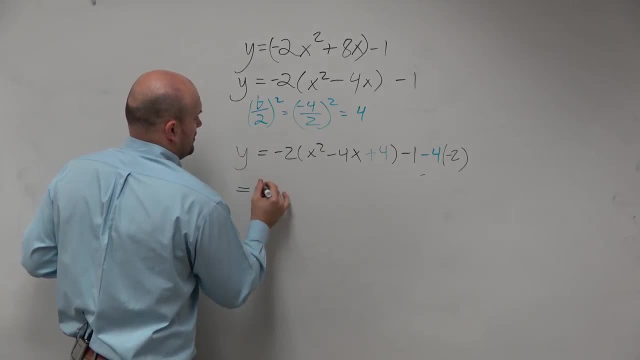 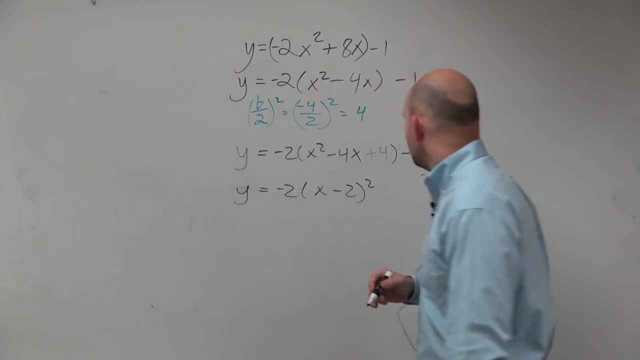 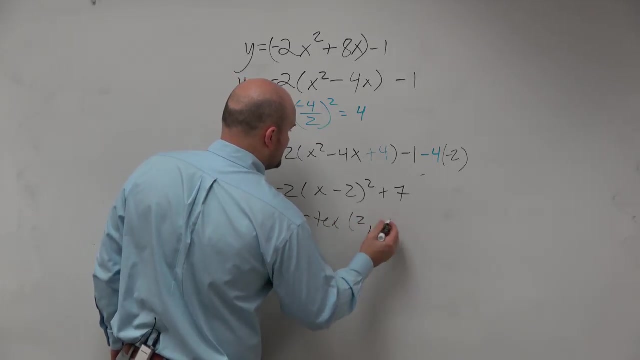 So let's go ahead and do that. So y equals negative 2 times x minus 2. squared Negative 2 times negative. 4 is positive 8 minus 1.. It's going to be a positive Positive 7.. Vertex is going to be 2 comma 7.. 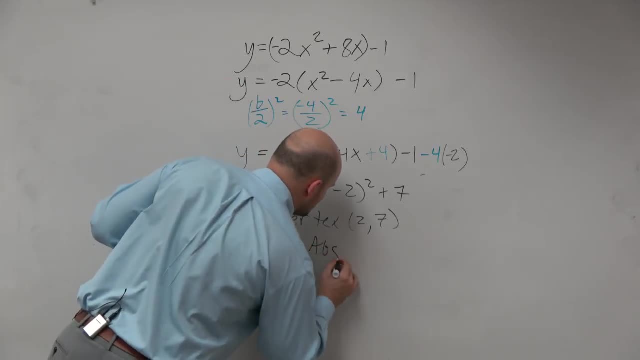 And you can see that's a negative, So it goes down. So therefore that's an absolute max. And again, guys, usually what we do,